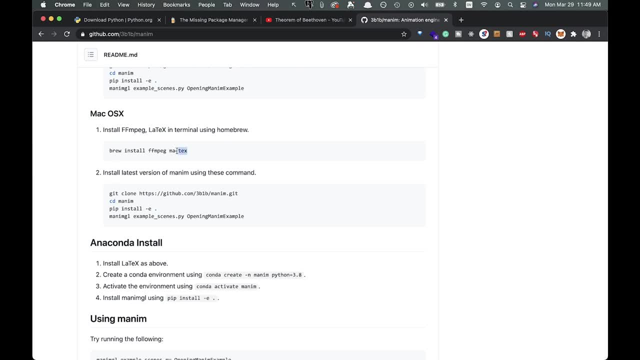 So basically you're going to install everything- Mac text or whatever latex version- you have FFmpeg- and then you're going to get clone the repo right here, Alright, and then from there we're going to CD into that and let's go check out the actual code. 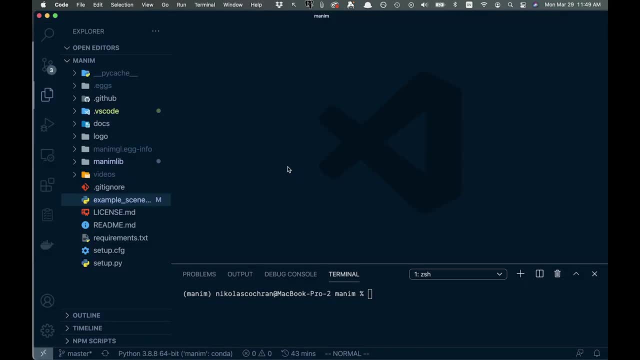 That you're going to get from there. All right, so this is what the package is going to look like. once you're CD into this and we have our Manum folder here, your videos, once you export them, will show up here, and then we just have this example scene which we're just going to work in today. 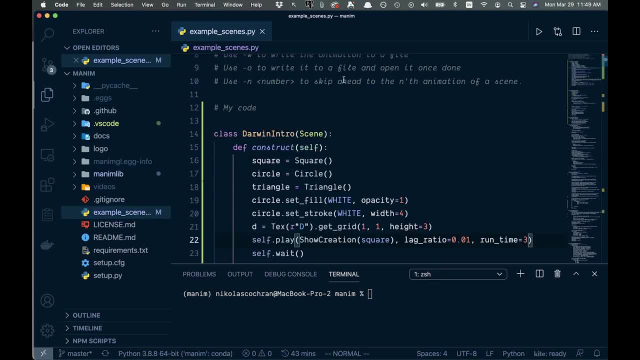 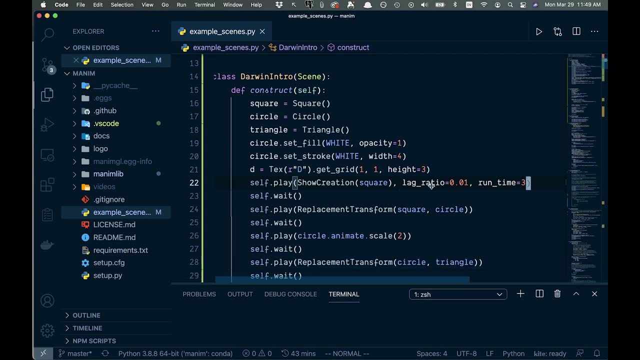 So if we click into this here, I created this intro here and that's what you would have seen at the beginning of this video, And it really took me almost no time at all. So it just kind of shows you how quick you can build out some simple animations. 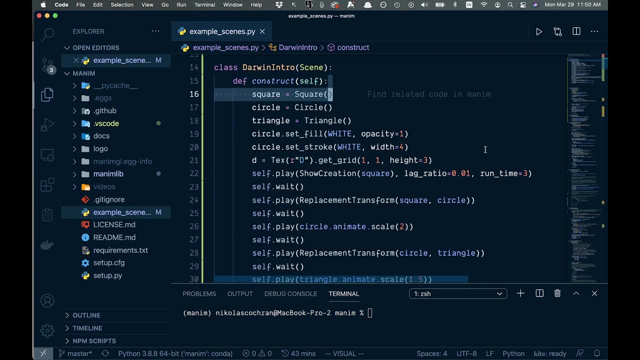 So we'll just go through a few different things. Definitely, check out the documentation, because it's fairly well documented, and I'll show you just a way more variety of things that I'll show you right here, But I want to give you a taste of what you can do. 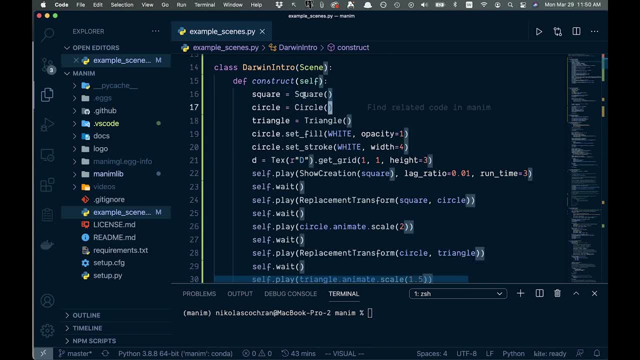 So first of all, you can create some shapes here. So you can see, I've created a square or a circle here, You got a triangle and use all those, And then you have these different methods so you can chain on all these different things. 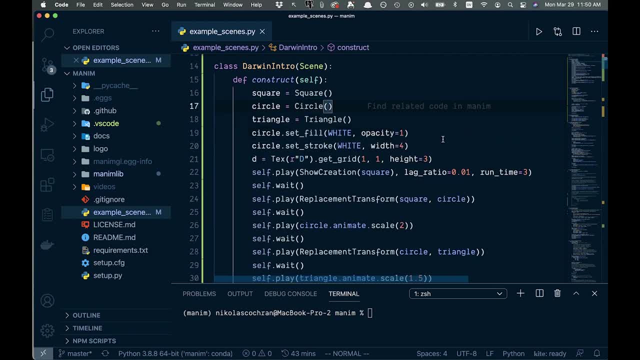 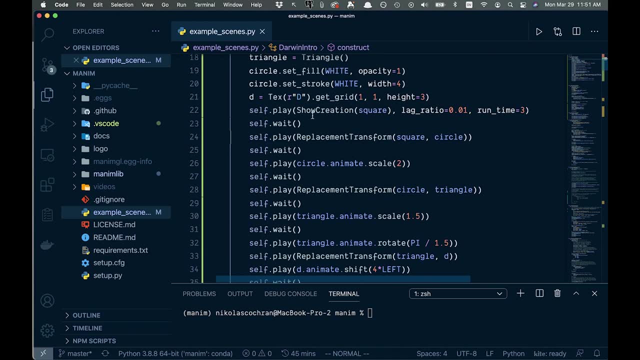 So, if you see, here we have the set fill, fill it with whatever color you pass in and an opacity, All right, And then, coming down here we can create some text. here We have this show creation which will actually run the animation. 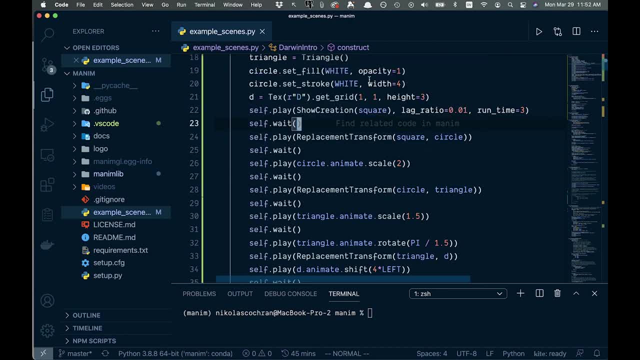 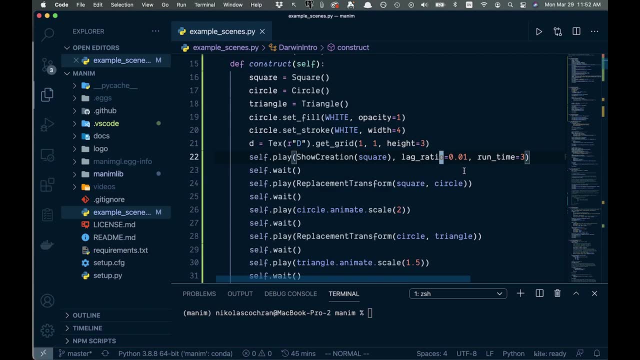 So it'll be at the end the outline, And then we pass in the square that we created up here, And then you have a lag ratio and then how long it takes to run it. So that'll be the speed of the runtime. 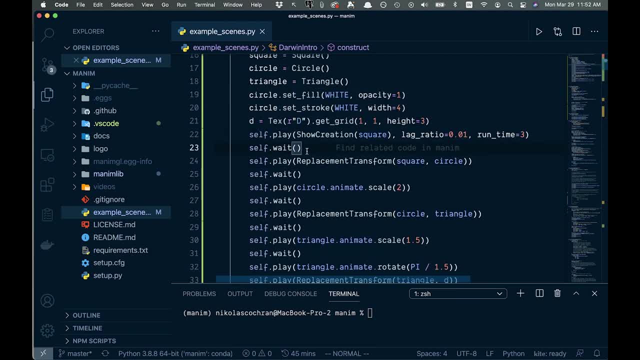 And then you'll have this wait method here and you can pass in a time there too. if you want to wait longer, you could pass in a two or or whatever. We got scale over here, and this is how you animate something, So you can animate this circle by just 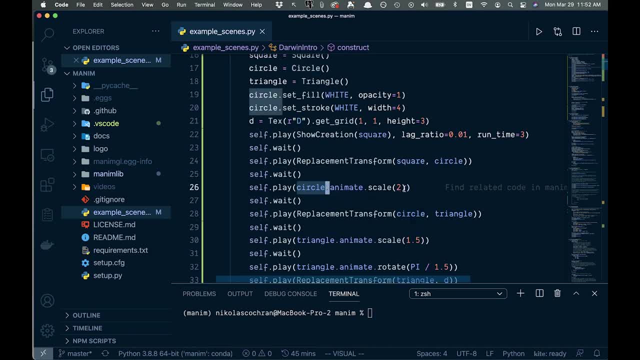 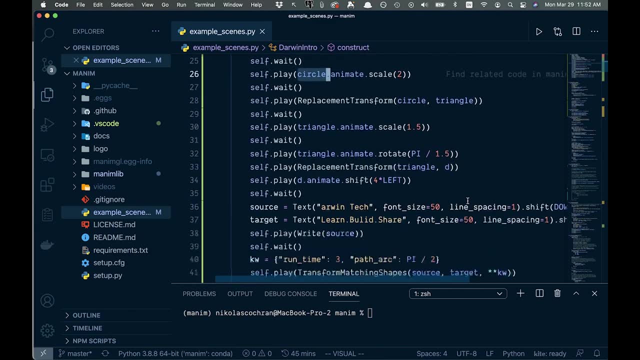 chaining on the animate method here and then scaling it by two. So we're going to animate here and scale it by two. Just some more things you can do. So basically, you can go through all these different things. We can just write out the text and I'll animate it. 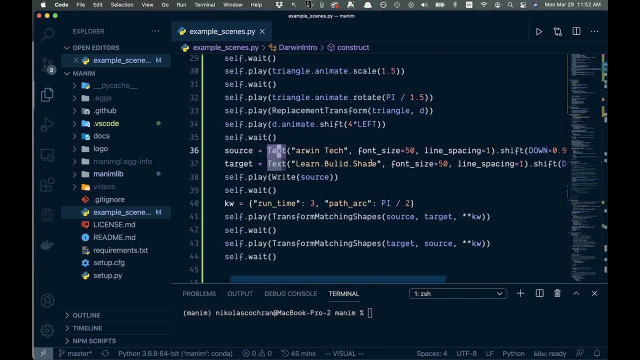 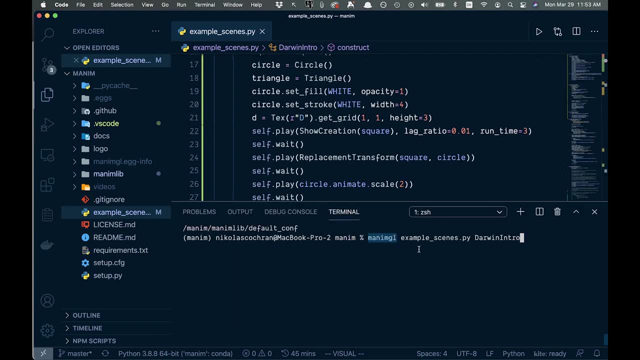 This is how I did the Darwin tech here anyway. So there's a ton of different stuff you can do, So let's run this again here. So in order to run this, we're going to be in our folder I'm going to call Manum GL and then the example scenes, which is this file here. 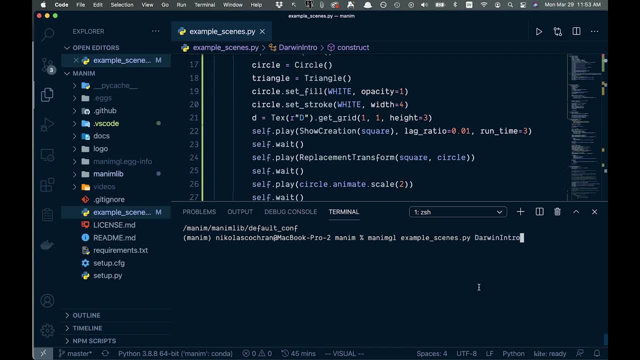 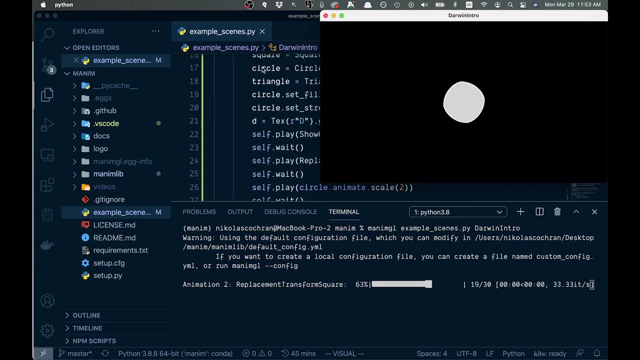 that we're in, and then the class name, which for us is Darwin, intro for this one. So let's run this again And you can see it's just going to animate And as we go it'll kind of run through this step by step. 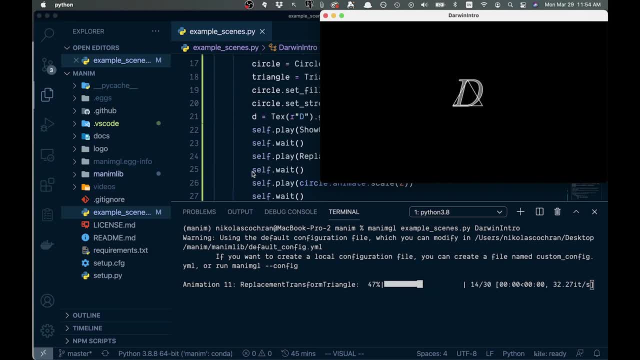 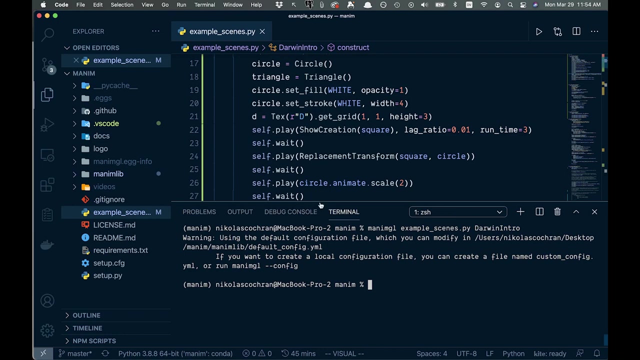 And all these transformations are happening at the same time. So so pretty neat stuff. So this isn't the greatest animation or anything, but it kind of gives you an idea of what you can do. OK, so let's check out some of these other ones. 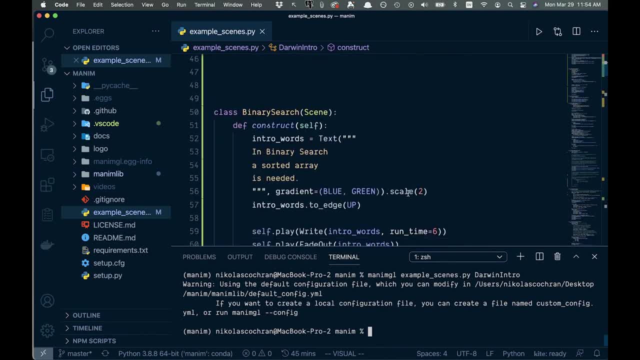 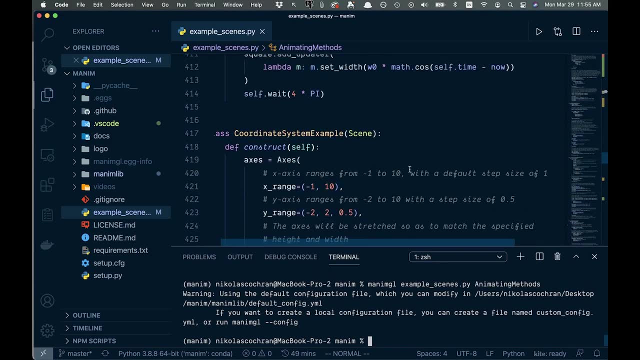 This example scenes is actually great. They give a ton of different examples of different things you can do. So if we scroll down here, let's check out another one. Let's check out this coordinate systems example here. So we'll just run this. 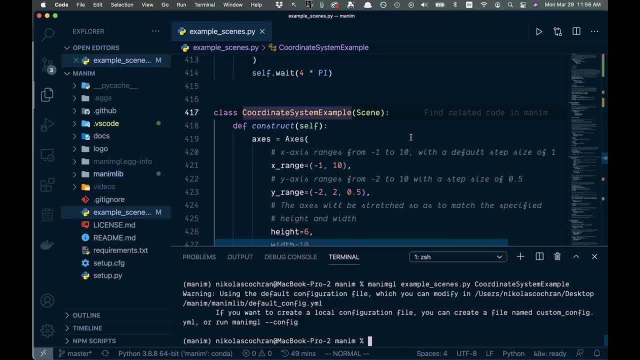 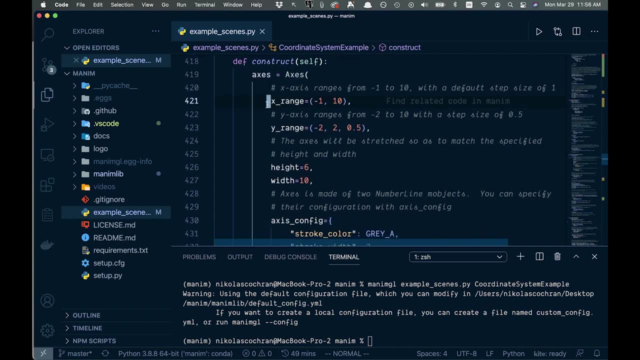 All right. So you can see how this is just super useful if you want to animate any sort of math functions or anything. So in this one we just came in, You create an axis here And you can create the X range and the Y range. 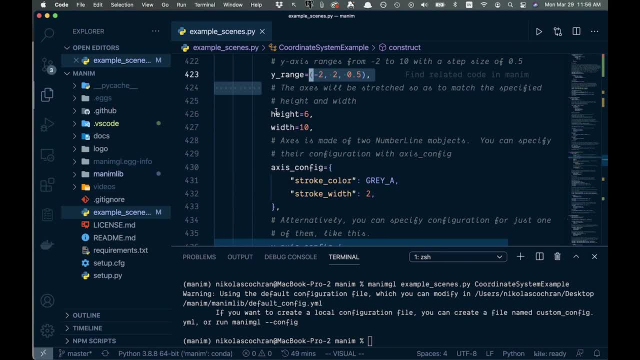 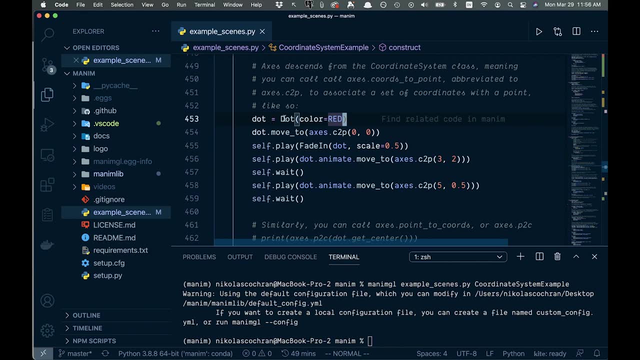 So wherever you are in the axis, and then you have a height and a width- kind of some styling here, All right, And then you create your dot. You can add a color. So this is just like the square or the triangle, the circle or any of those dot is one of them. 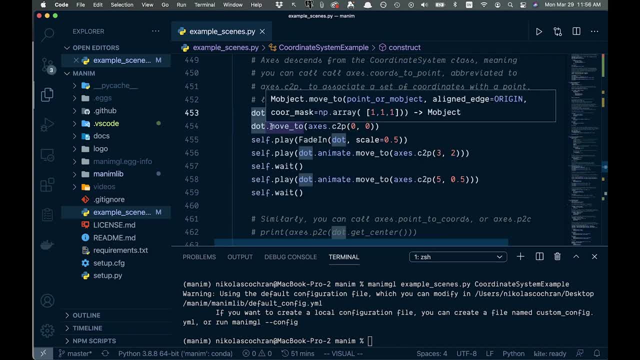 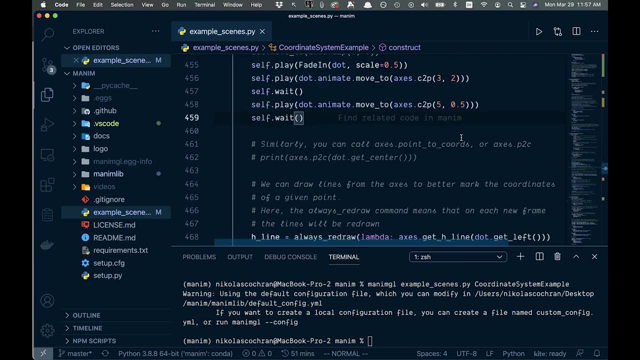 So you can add that, and then you can use this method, move to- to actually move the axes and the dot along it. So that's pretty nice, And then again we're just animating the dot, Basically just some pretty cool animation stuff you can do quite easily. 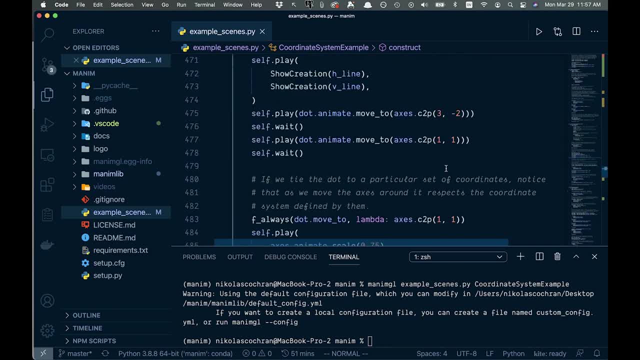 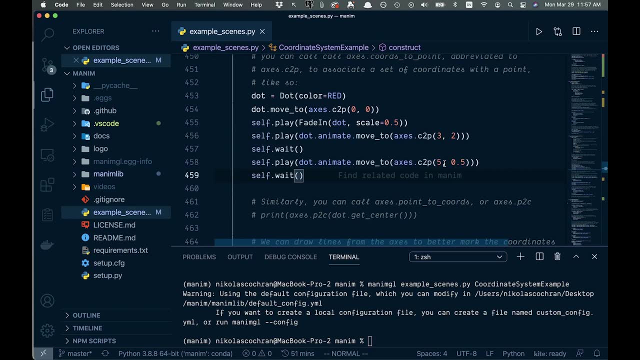 And you can see, this isn't like a super long class or anything. It's, I don't know, maybe 50 lines or something, not even So, it's quite easy to get this going, All right, So let's just show you a couple more. 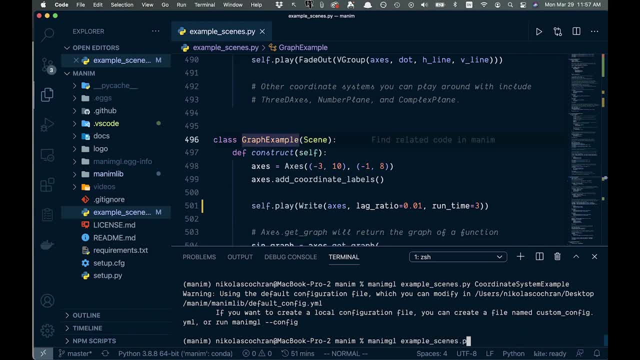 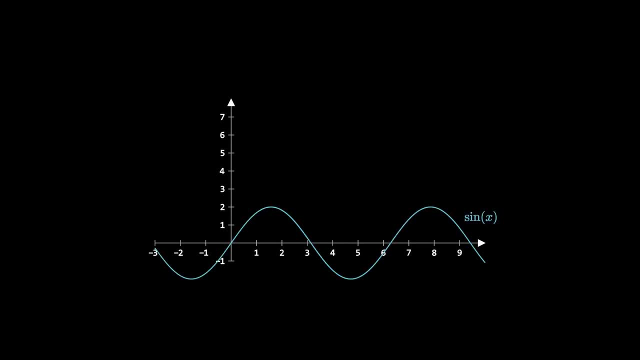 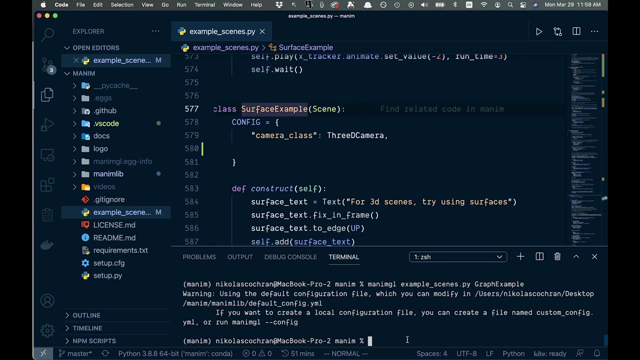 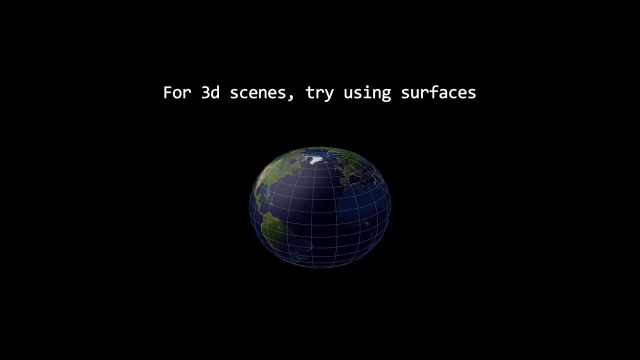 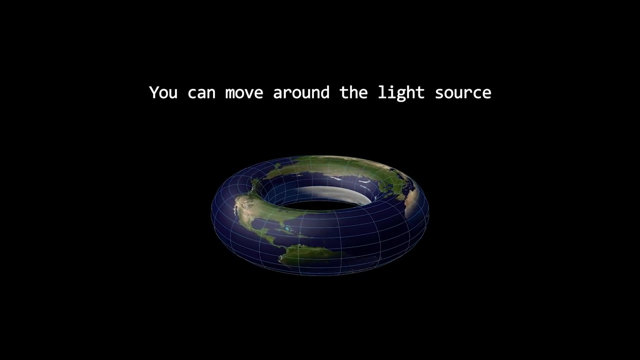 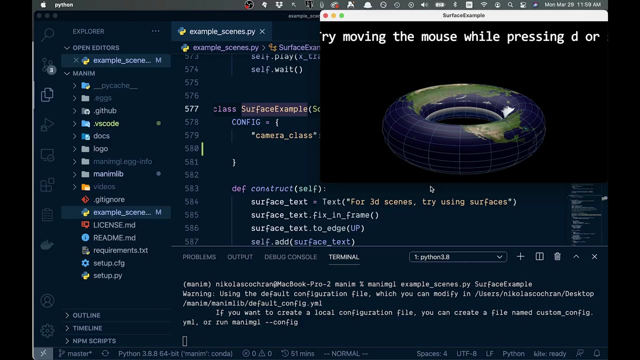 Let's maybe try this graph example, All right. And then there's actually you can do a lot of 3D stuff with this too, which is kind of cool. Let's run the surface example here. So so this example is just kind of blowing my mind a little bit and it's actually kind. 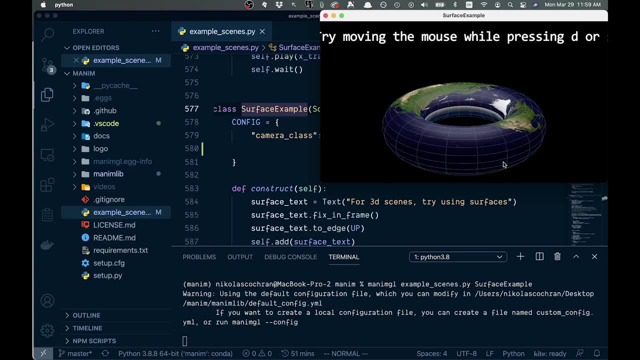 of interactive. So if we press D we can actually move around with our mouse here and actually change the view of this. So that's pretty insane right there And kind of the crazy. The thing I think about all this is, if you come in here back into our surface, 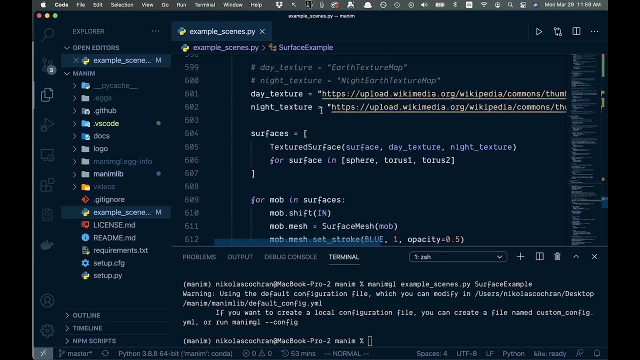 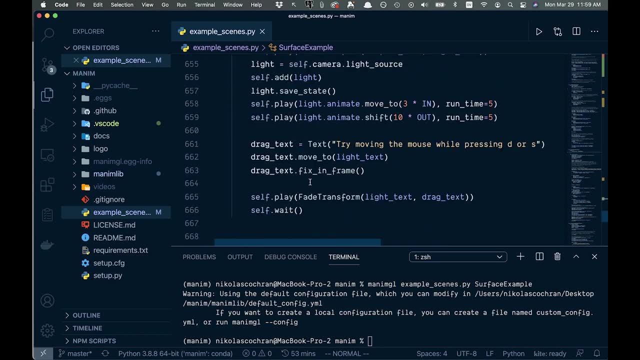 example, if we come into this example, it's not a huge class here, Like there's just not that many lines of code in order to create this Something you would think would just be crazy tough to to to create. So I think that is pretty, pretty awesome. 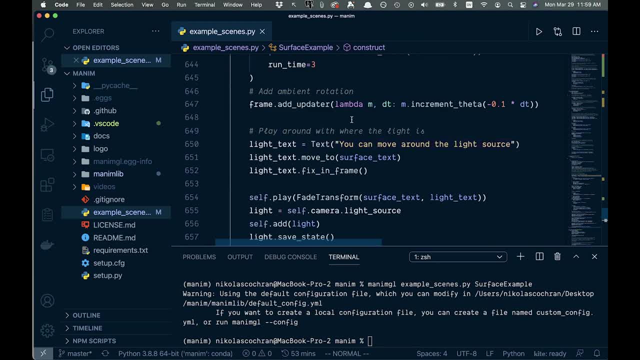 So we're not going to go too in depth in any of this, but just check out the docs and play around. If you play around for like 20 minutes, you'll kind of get the hang of it, and then you can just look up whatever you want. 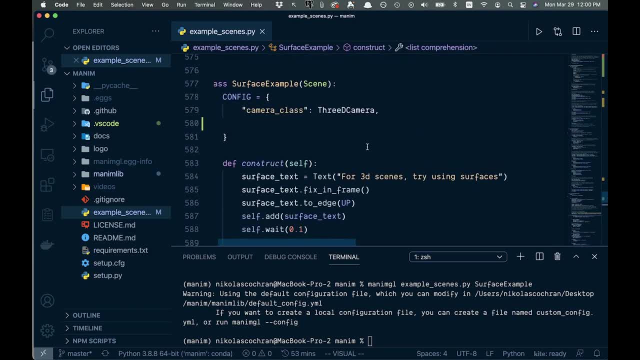 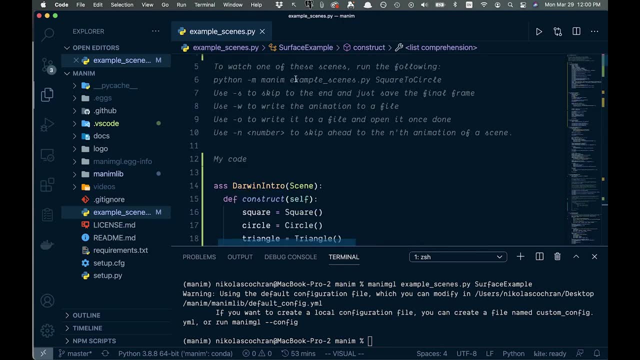 to do, basically, And kind of chain everything together like that. The last thing I want to show you is, if we come back up to the top of this file here, I would just go through all these example scenes also, if you were, if you're. 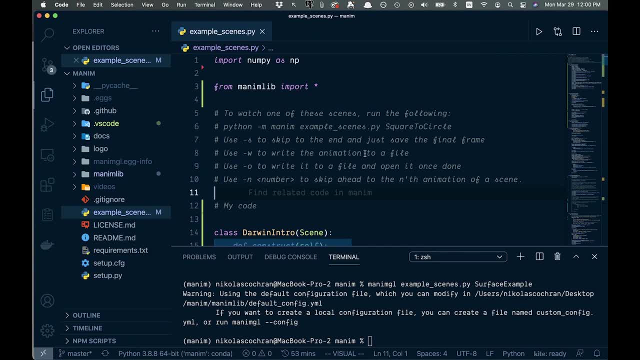 interested but a lot of these flags we can add, and S will skip to the end, W will write to to the file and then O will write to a file and open it. So if we want to actually get the video from that and write that to a file, 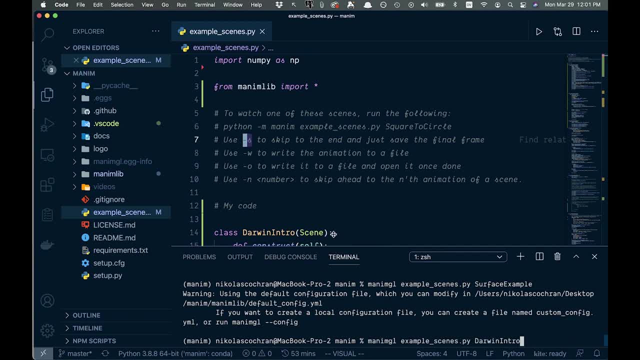 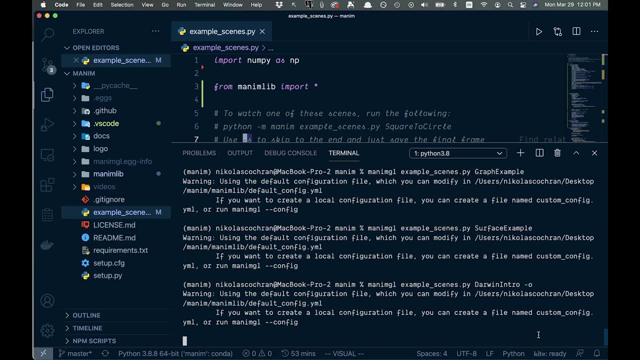 we can come in here, I'll go Darwin and show the one I created, And then we can just go: oh, like this, And you'll see that I'll actually write it to a file. All right now, when it's done, you can see, it just pops open here and we can just